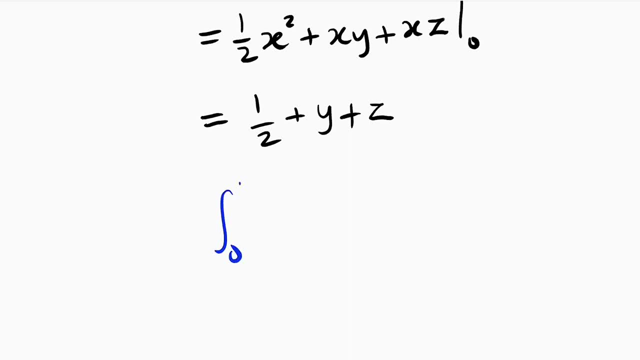 So we have the integral from 0 to 2, of 1 over 2 plus y plus z. with respect to z. Now we are going to integrate: This is equal to: this is constant. this is constant. We are going to multiply them by z. So we have 1 over 2 z plus y, z plus this is: 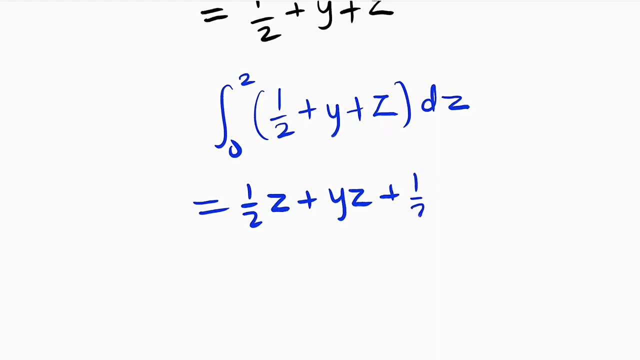 the function. If you integrate it, you have 1 over 2 z squared, our boundaries from 0 to 2.. All right, wherever we see z, we substitute by 2.. This is equal to 1 over 2 multiplied by 2 plus 2y plus 1 over 2, 2 squared. We don't have to substitute the lower bound because it is going. 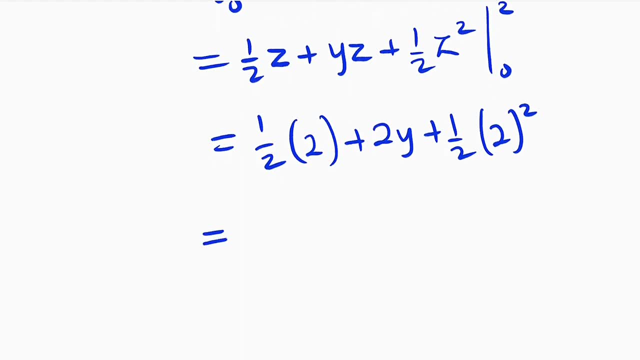 to make everything 0.. So let's simplify: Half times 2 is 1 plus 2y 2 squared is 4.. 4 multiplied by half is 2.. So we have plus 2 here. If you further simplify, you're going to obtain: 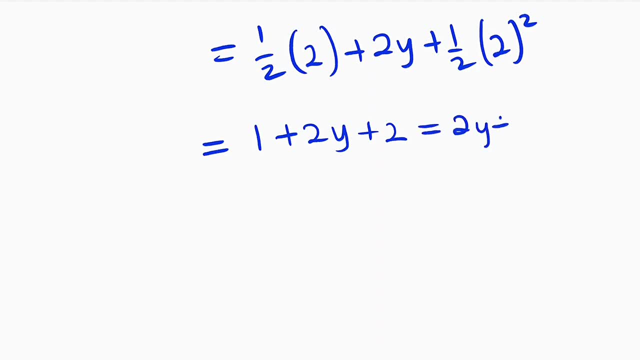 3 plus 2y or 2y plus 3.. So 2y plus 3 is going to be the last function we are going to integrate with respect to y. Which is this We are going to integrate with respect to y? 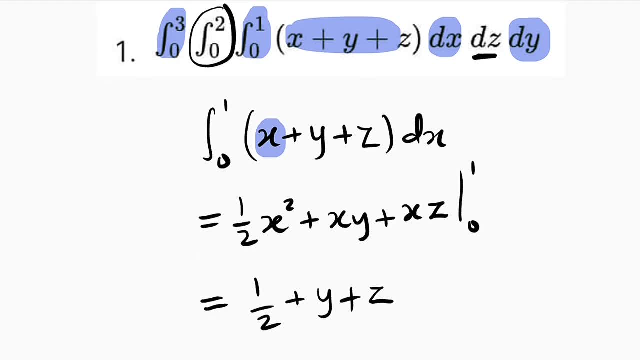 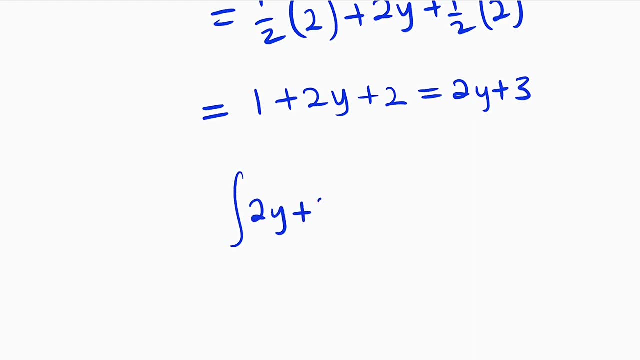 using the first definite integral from 0 to 3.. So, lastly, we have the integral of 2y plus 3 from 0 to 3.. to 3 dy. Alright, let us first of all integrate 2y. If you integrate 2y, you're going to obtain: 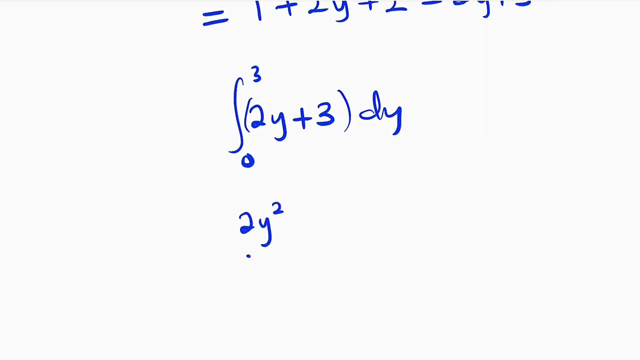 2y to the power of 2 divided by 2 plus 3 is constant. We are only going to multiply it by y, Our boundaries from 0 to 3.. This is equal to 2 will cancel 2.. All we have is y. 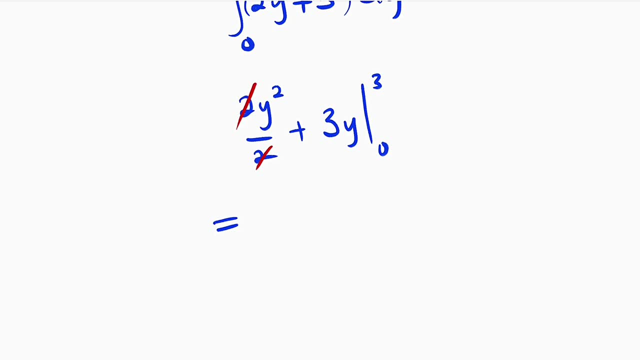 squared, We are going to substitute y equal to 3.. So we have 3 squared plus 3 multiplied by 3.. 3 squared is 9 and 3 times 3 is also 9.. Finally, we have 9 plus 9 equal to 18.. Therefore, the first problem is equal to 18.. If you integrate the 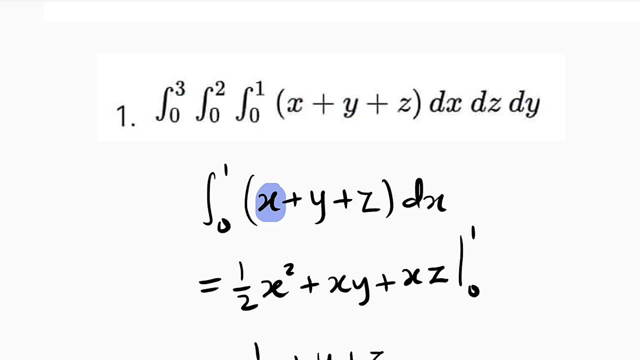 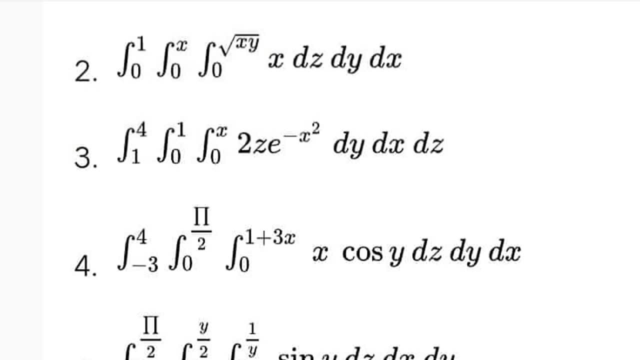 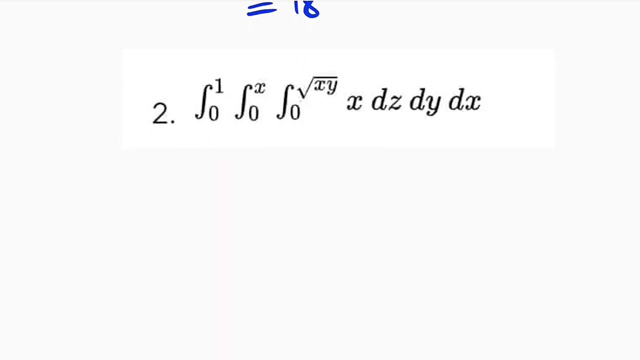 whole of this function with respect to x, z and y, you're going to obtain 18.. So now let us take the second one, which is a definite integral of only a function: x with respect to z, y and x. Alright, here is the problem. Let us start with this. So we have the integral from 0. 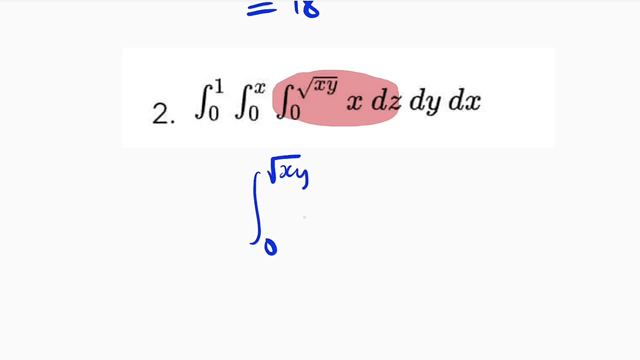 to root x, y of only x, dz. Our function is x, but we want to integrate it with respect to z, So all we have to do is to multiply it by z, So this becomes x, z, y, y, y, y. 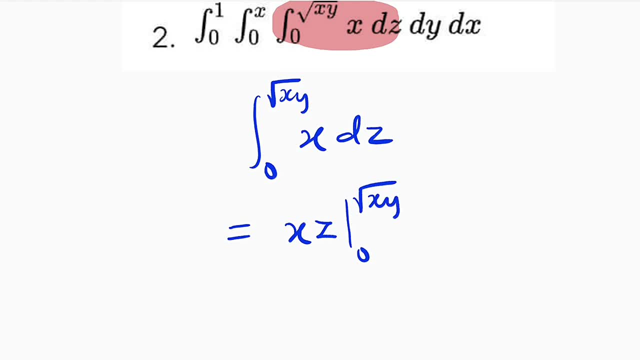 from 0 to root x- y. So wherever we see z, we replace it with root x- y. So this is equal to x multiplied by root of x- y. We don't have to substitute the lower bound, because it is going to make it 0.. Alright, let us further simplify this. Remember that from: 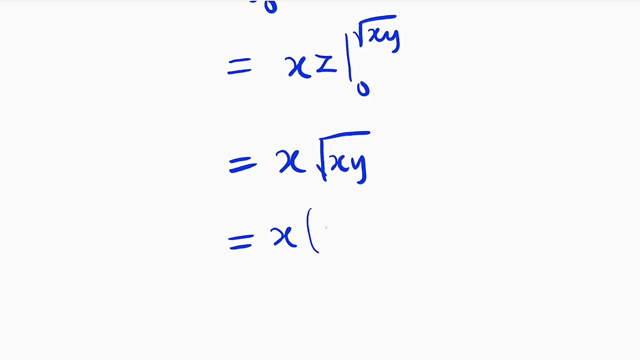 the law of indices this can be written as x. So we have to multiply by x to the power of 1 over 2, multiplied by y to the power of 1 over 2.. You know, naturally this x has a power of 1.. So if you multiply x by x, you're. 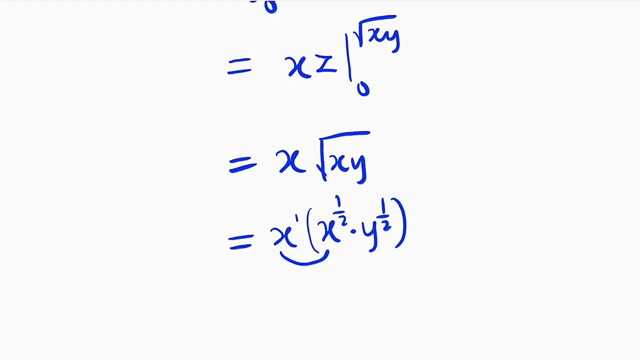 going to obtain x to the power of 1 plus half, which is 3 over 2.. So, finally, this is equal to x to the power of 3 over 2, multiplied by y to the power of 1 over 2.. 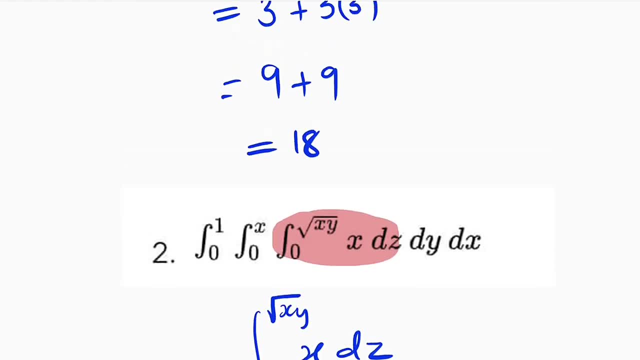 So this is our new function and we are going to integrate it with respect to y, from 0 to x. So we have, from 0 to x, of x to the power of 3 over 2, multiplied by y to the power of 1 over 2 with respect to y. 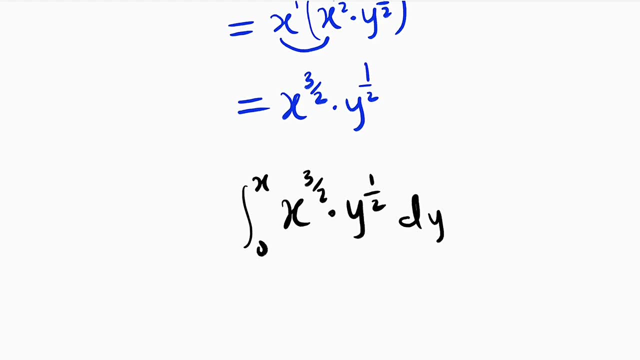 So we have to integrate it with respect to y and we are going to treat this as constant. So this becomes x to the power of 3 over 2 multiplied by. if you integrate this, you add 1 to the power, it becomes y to the power of 3 over 2, and you have to also divide by. 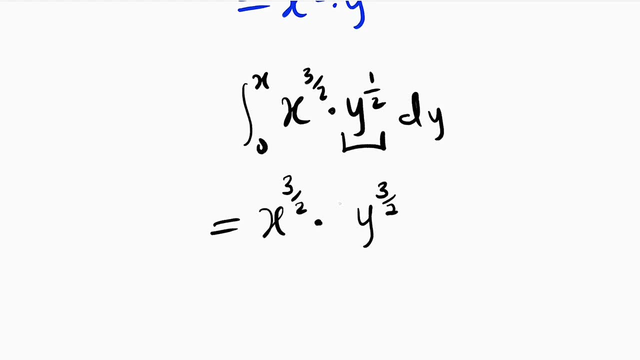 the power, which is the same thing as multiplying by the reciprocal 2 over 3.. our boundary from 0 to x. Alright, let us substitute the boundary- This is equal to x, to the power of 3 over 2 multiplied by 2 over 3.. y is x, so we have x to. 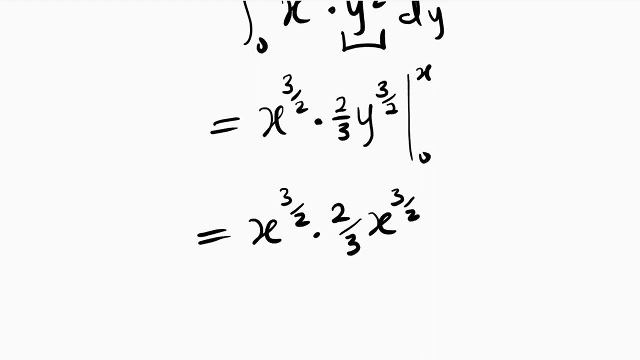 the power of 3 over 2.. We don't have to substitute the lower bound, because this is going to make everything 0.. Now let us further simplify. We can bring 2 over 3 back. Then we multiply by x to the. 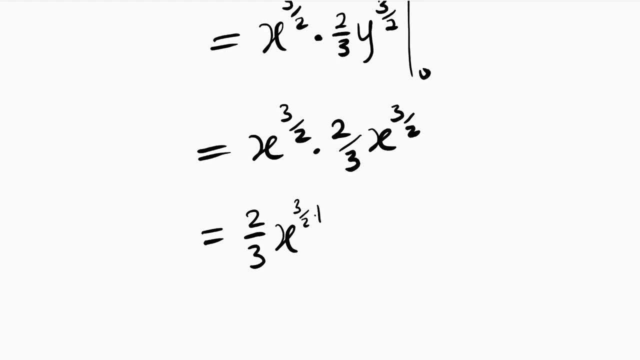 power of 3 over 2 plus 3 over 2 using one of the laws of indices, And 3 over 2 plus 3 over 2 is the same thing as 6 over 2, which is the same thing as 3.. So this is equal to 2 over 3. x to the power. 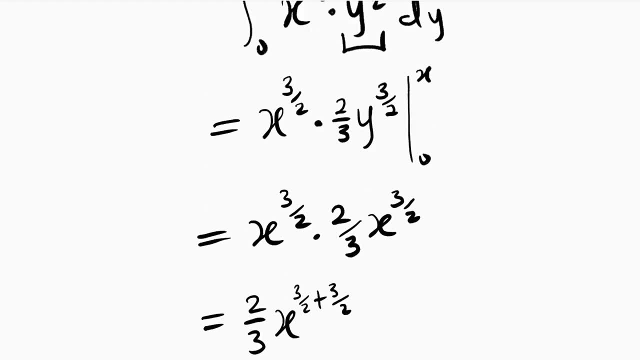 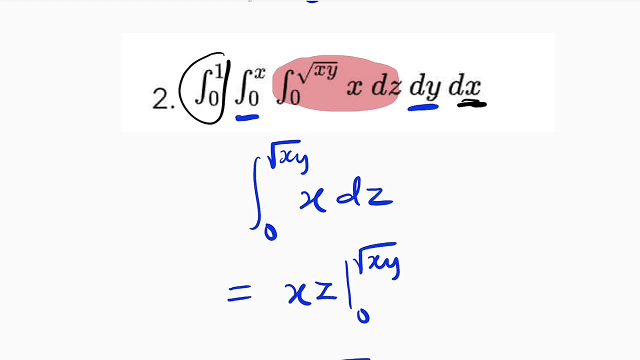 of 3.. This is our last function that we are going to integrate with respect to x. You can see the last one here, from 0 to 1.. So we have the integral from 0 to 1 of 2.. We can bring it out 2 over 3.